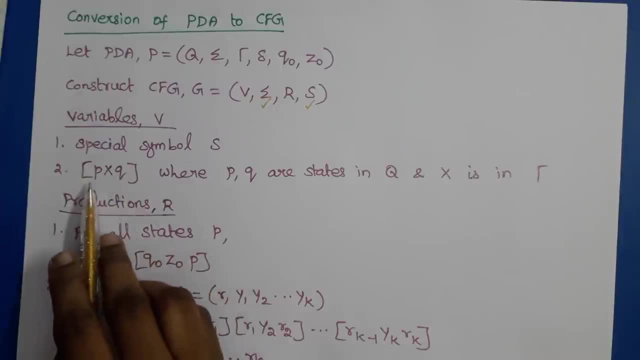 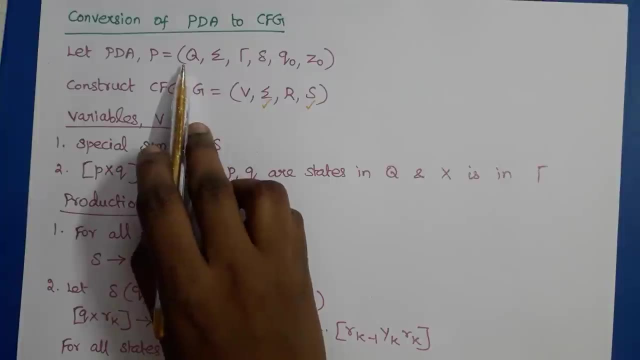 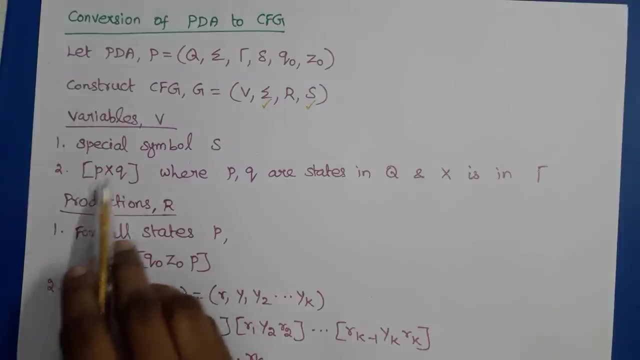 using the square bracket. so within the square bracket we have to write p, x, q means p and q, where p and q are the states in q. for example, if pda has q, naught, q1, q2, then we have to write form all the variables with q, naught, xq, naught, q, naught, xq1, like that. 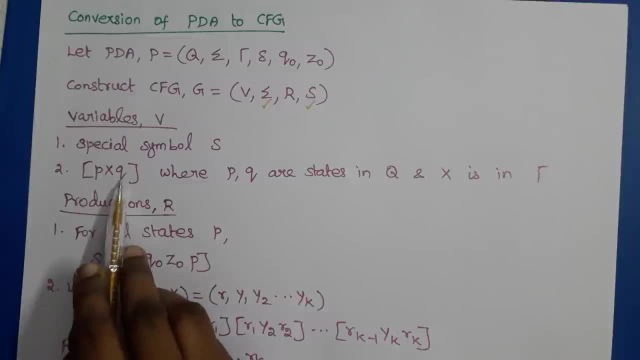 so where this p and q- first symbol and last symbol are the states in q and the middle symbol x is, is the x is the stack symbol. okay, so first symbol and last symbols are the states. middle symbol is a stack symbol, so this is considered as a single variable. 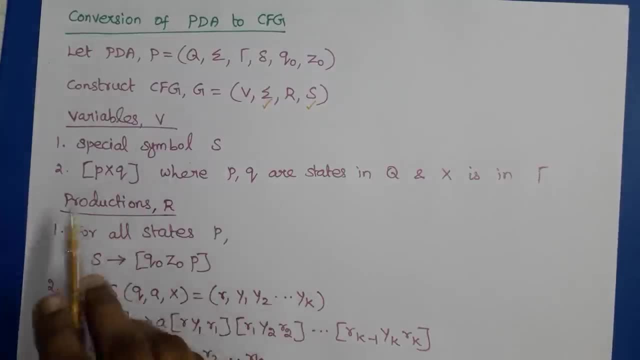 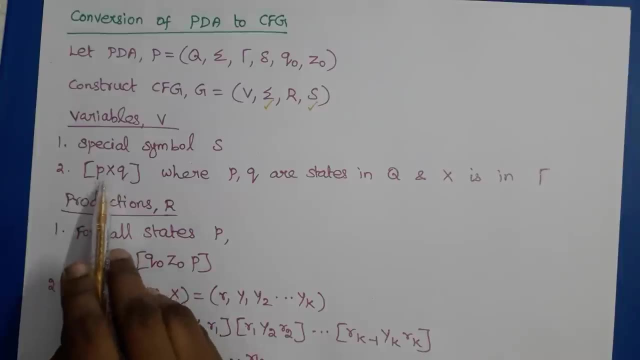 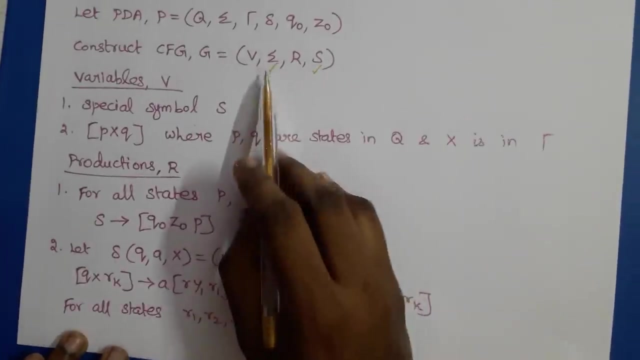 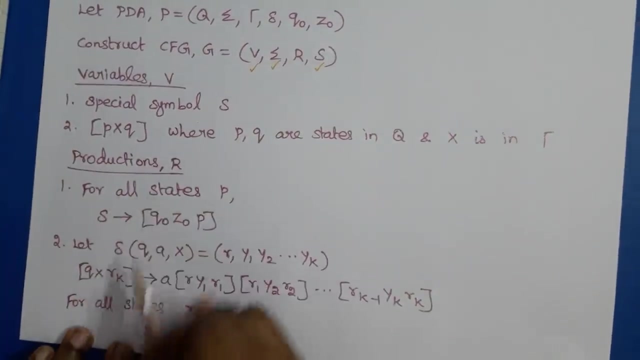 okay, yes, is considered as one variable. other variable is a single variable must be formed for all possible combinations of the states and all possible combinations of the stack symbol. So we have to construct variable like this, Then productions that, so variables formed by following these two rules, then we need to form the rules, So there. 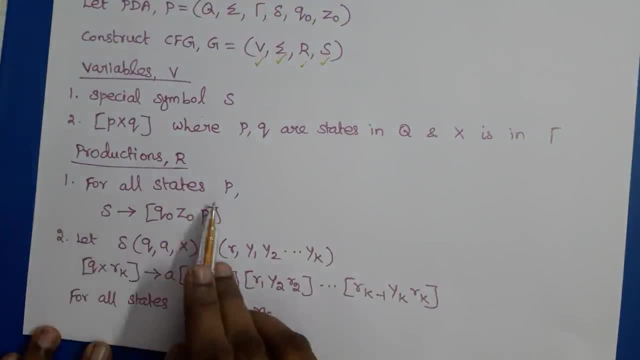 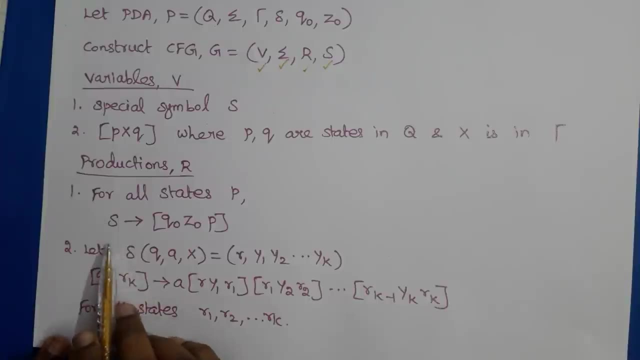 are two rules. So first one is for all states P in Q, for all states P in this capital, Q, we have to write the set of productions like this: S tends to: that is the start symbol of the grammar S. Start symbol of the grammar S tends to: Q0, Z0, that is, within square bracket. 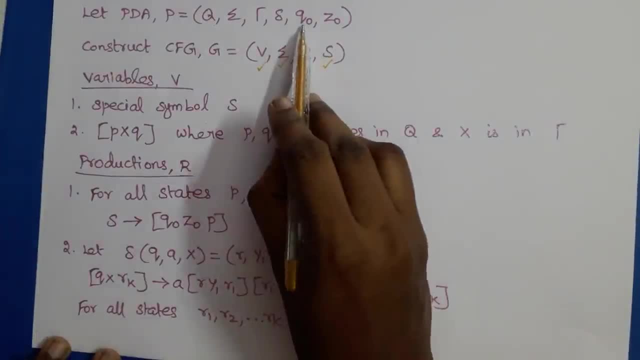 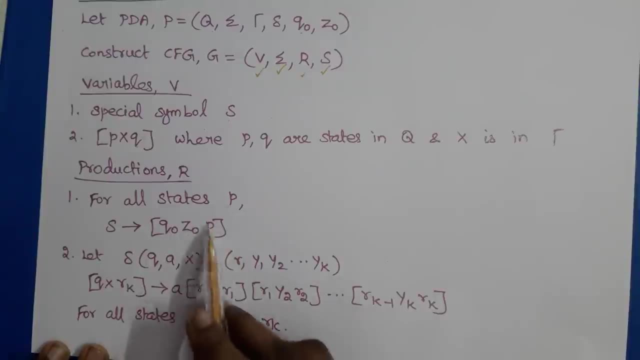 it is a variable, single variable. So within square bracket the start state of the PDA, Q0. starting symbol of the stack: Z0. then for all possible combinations of P we need to write this. So, for example, if the Q has P0, then we have to write the set of productions. 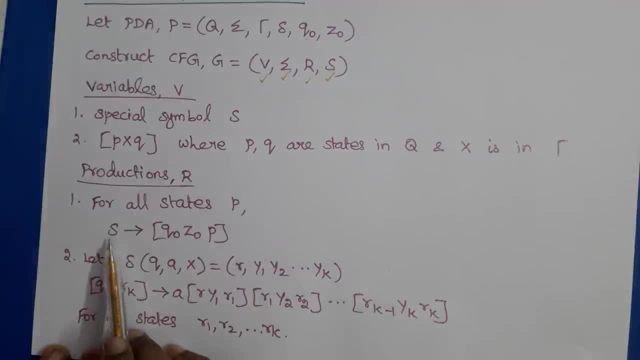 P and Q. There are two states. P and Q means then the productions are S tends to Q0, Z0, P, then S tends to Q0, Z0, Q. So this rule must be written for all possible combinations of this symbol. So first two symbols are Q0- Z0 only, and that means start symbol of the sorry. 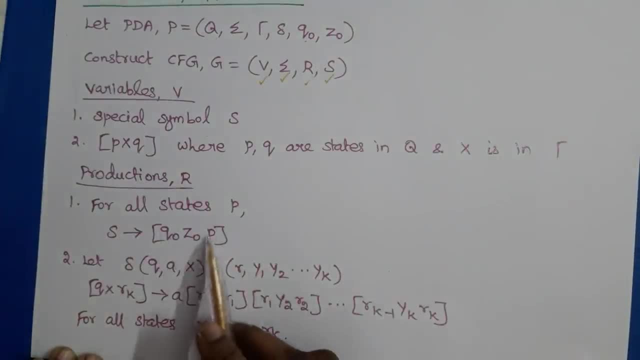 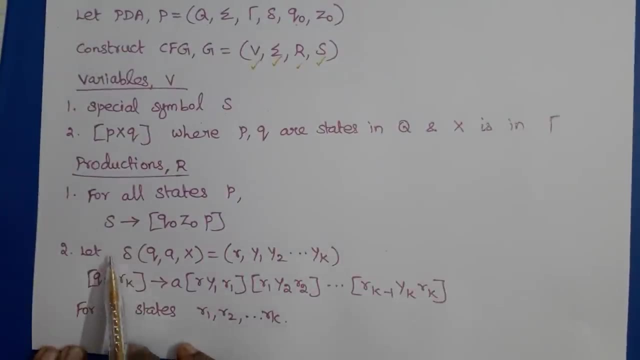 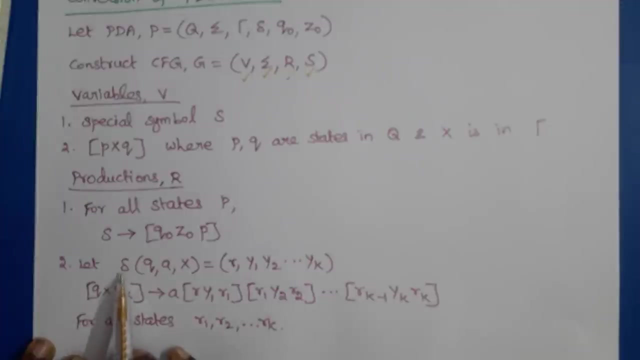 starting state and starting stack symbol, then this state. this must be written for all states in Q. Then for the second rule should be written for all the transition function of the PDA, for all transition function. we have to follow this rule. So consider it has a transition. 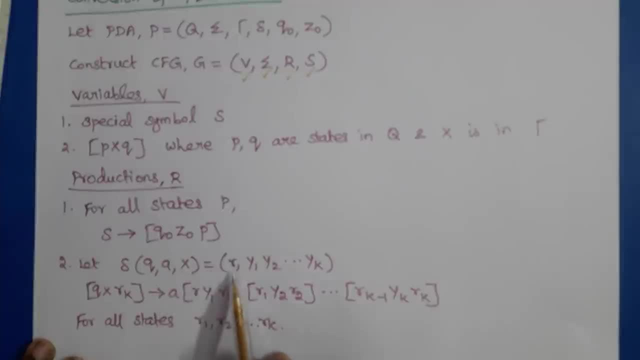 like this del of Q comma, A comma X equal to R comma, some K number of symbols: Y1, Y2, up to YK. that is, the current state of the PDA is Q. current input symbol is A. top of the stack is X and the next state is R. 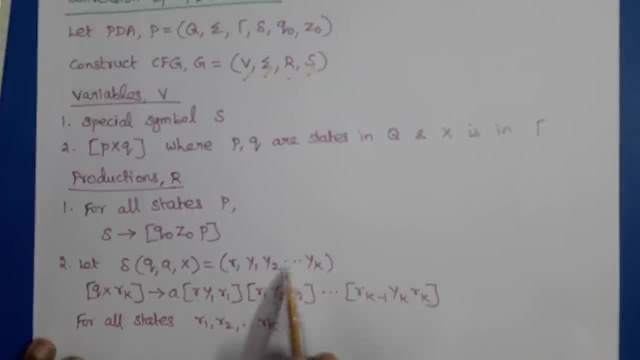 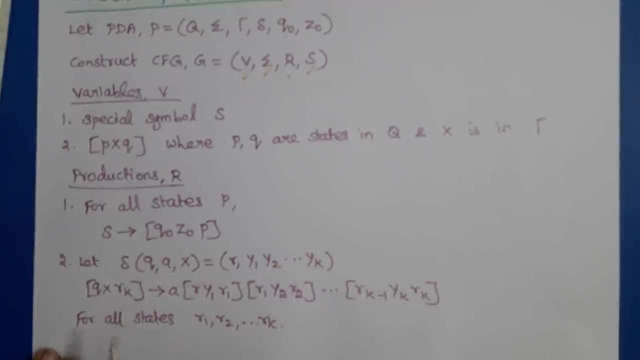 And this Q is the string of the string replaces symbol X on top of the stack. that is push. operation means then how to write the production for context free grammar. if PDA has a transition function like this, then production we have to write like this, So a variable can be formed. 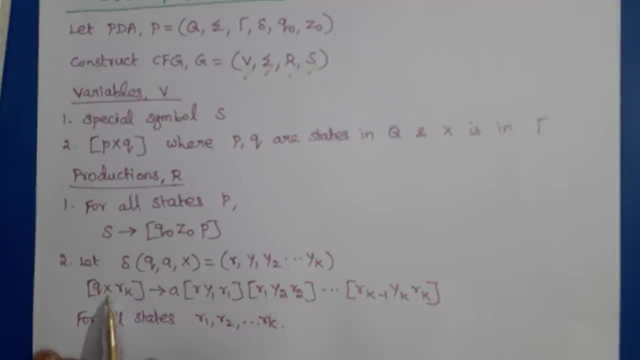 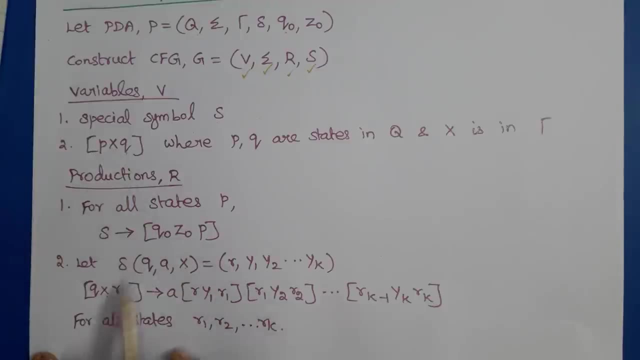 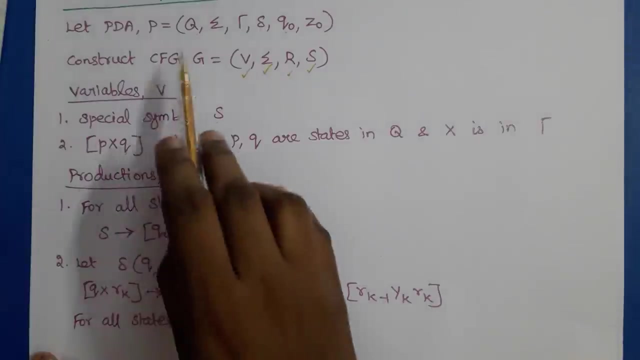 by combining this: Q, X, because variable can be written like state stack symbol state. So this q x and r k, and this must be written for here. k symbols are there, so we need to use k. k variables must be written here. so assume that the set of states are r 1, r, 2, dot, dot, dot, 2, r, k. 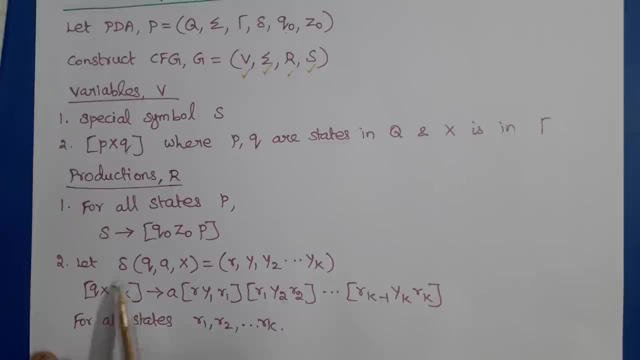 k number of states are there, then for all possible combination of the state we need to write this rule. so q x 1 is written here. so q x, this r k tends to q x, this q and this x. then r k tends to the terminal symbol a. then we have to write k variables here. here k symbols are there, so k. 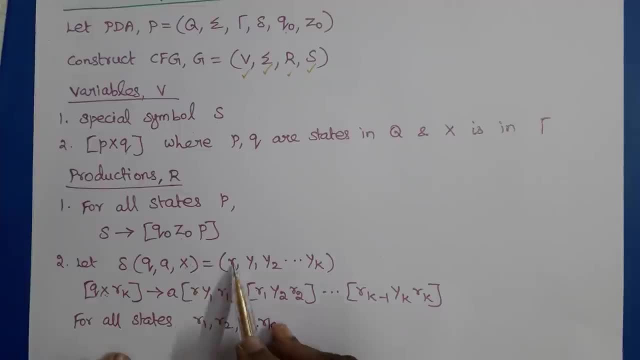 variables should be written. so this r should be written first, so r and y 1, then the new state r 1 and whatever state written here is written here. so this r and y 1 are written here, this is written here, so this r here, that must be written here also. so r1, then the next stack symbol, y2, then r2, then the next. 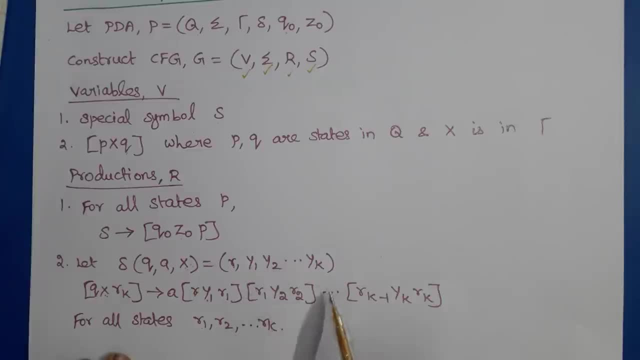 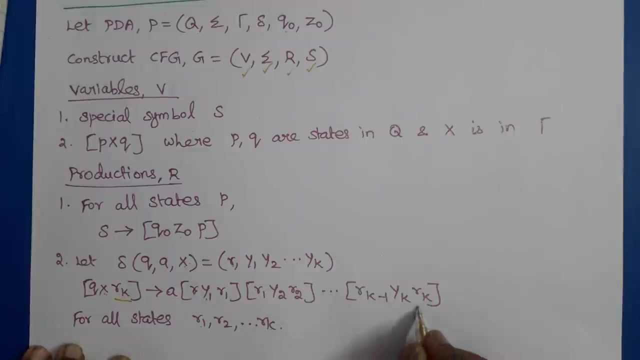 variable must be r2, y3, r3. okay, likewise we have to write. so the final symbol is here: r1 means y2, r2 are coming, so that rk minus 1, yk, rk. so this and this must be same in every production, this start state- sorry, current state- should be written here and top of the stack: okay, current. 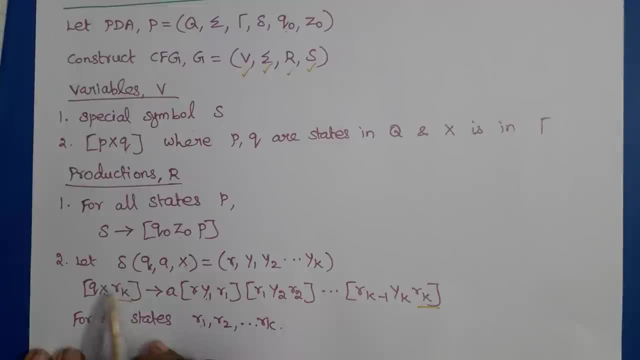 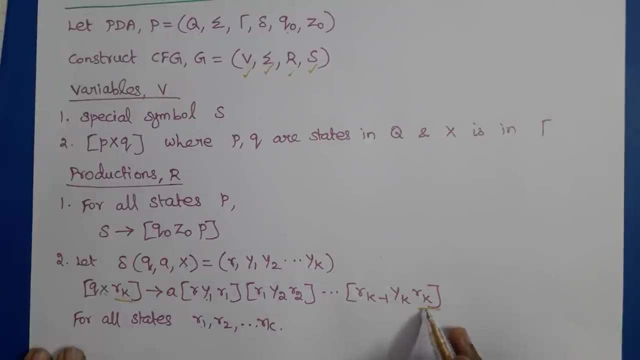 state top of the stack and a state. this must be. this rule must be written for all possible states. so here rk is written, means the final state state. here also the final symbol should consist of rk at the end. so this and this must be equal. and in the right hand side, after the production symbol, in right side we have to write the: 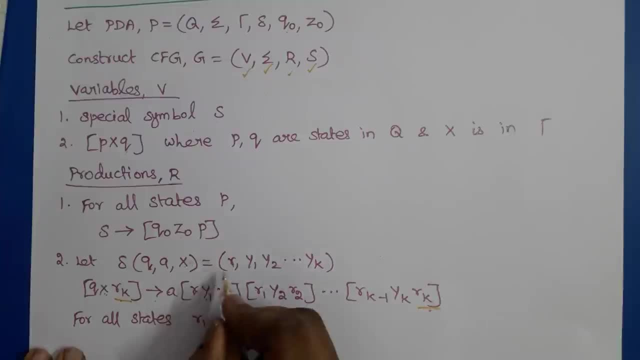 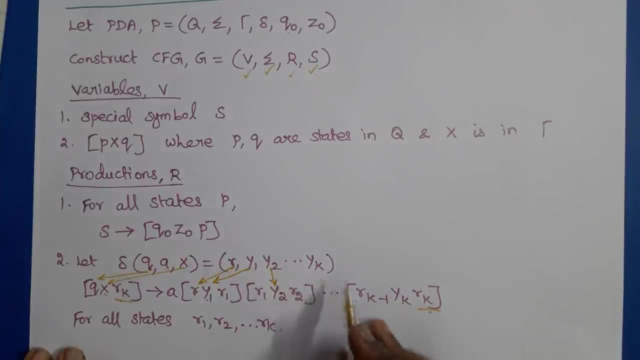 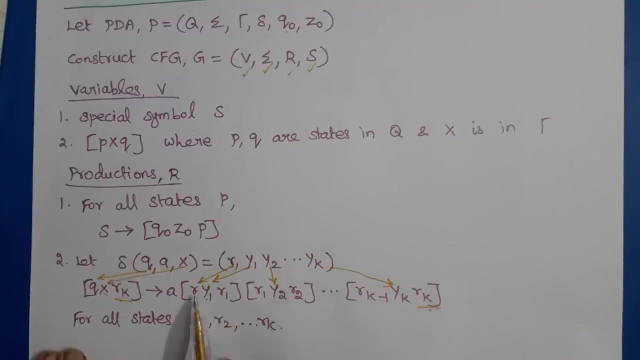 terminal symbol here, then this r. this r should be written okay. so this q, this x and this rk and rk should be equal. then this y1 should be written here, this y2, y3, up to y, k. so these symbols- these are the stack symbols- must be written in the middle part, and this r should: 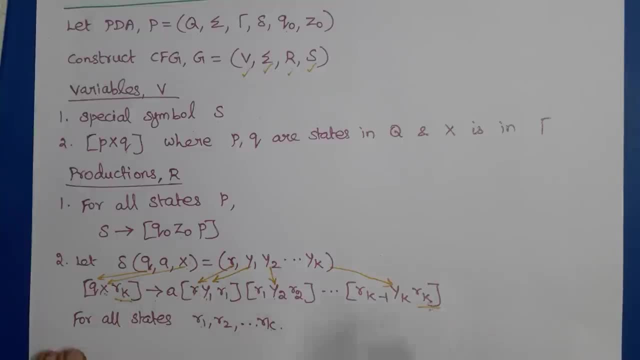 be written over here. the first symbol and final symbol must be equal. first state, this state and the final state. this should be equal and in the middle portion we have to write: whatever state is written here, we need to write it here. so: r2, r2, r3, r3. likewise, we have to write so if two symbols 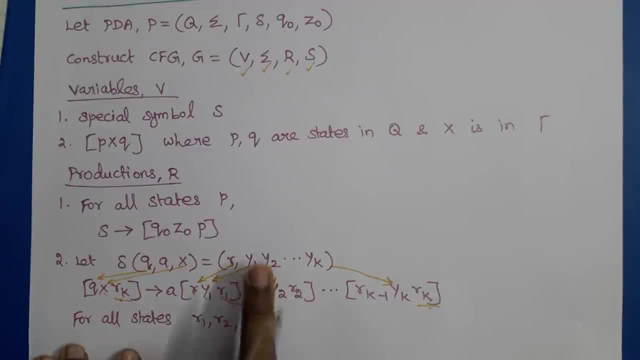 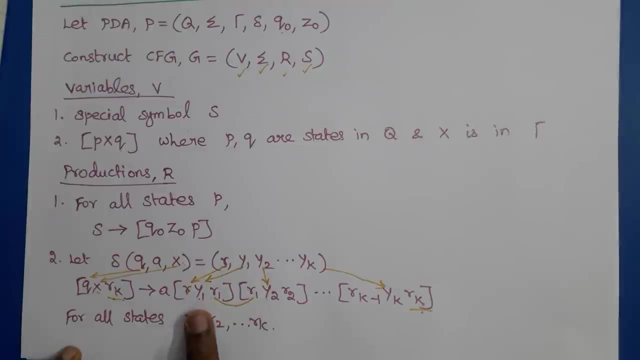 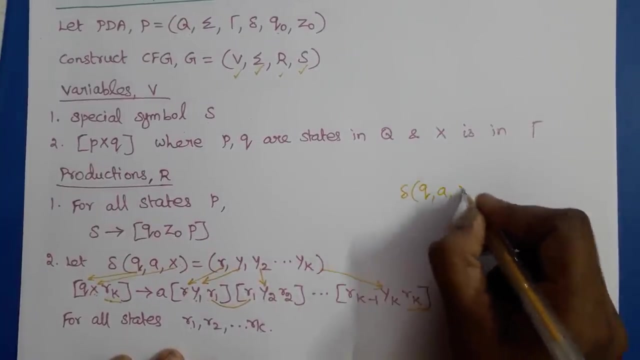 are given here, then two variables must be written here. one variable is written, then one- sorry, one- stack symbol is written here, then one variable should be written here. so sometimes this may be epsilon, for example del of q comma, a comma. x equals r comma, epsilon. so in this case we have 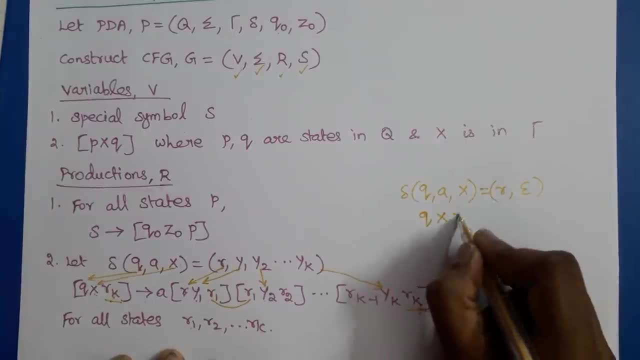 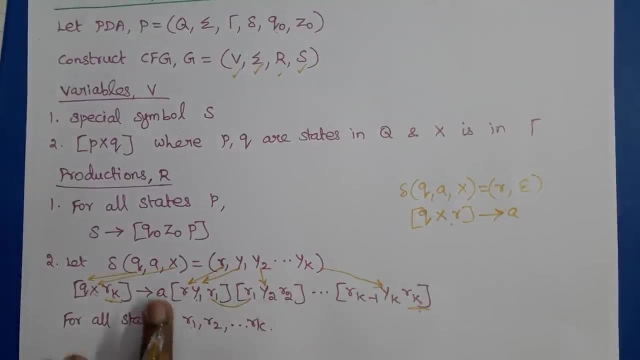 to write q x, r, q x. this r tends to a and this is the final state. so this is the final state. k- it has only one production, but this should. this must be written for all possible combinations of the states. okay, in the example we will see that. so for the k, more than one symbol. 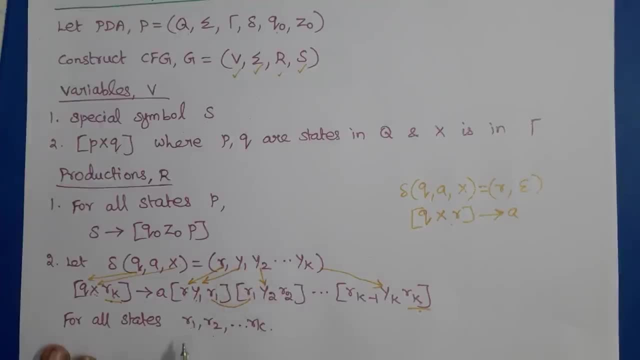 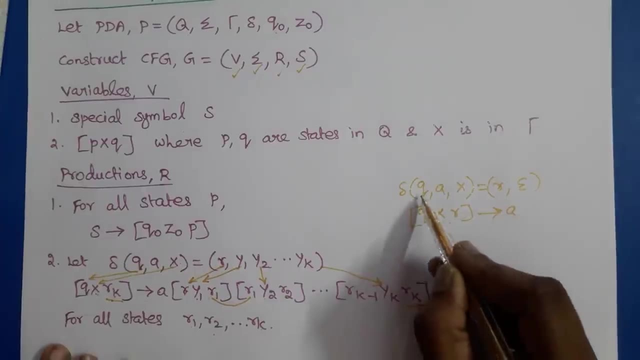 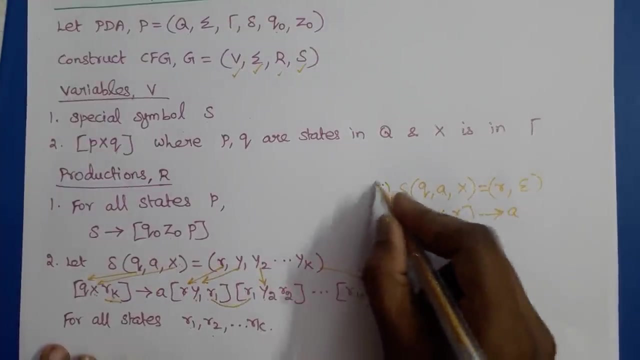 one or more symbols. we have to write the rule for all possible combinations, but here epsilon is given, then we need to write only one production by combining q x, r, then production symbol, this a should be written. this is second form. third form is sometimes this: a may be epsilon, so del of. 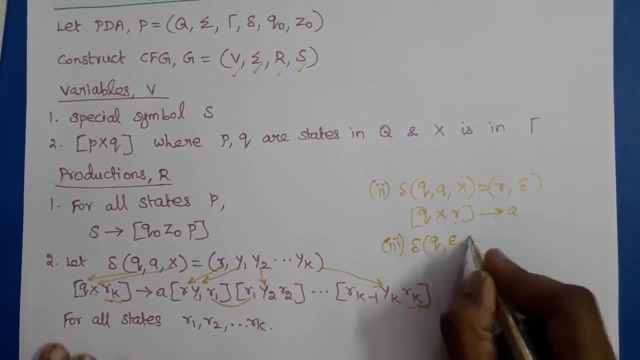 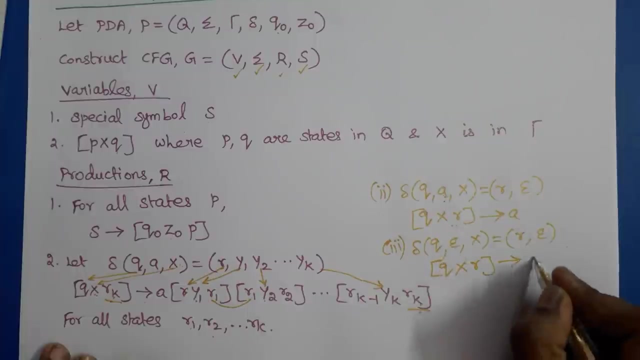 both a and here epsilon. so epsilon x equal to r comma epsilon. so here and here both may be epsilon. so in this case we have to write q x. this r implies this epsilon. okay, so these are the three. so here one or more symbols may come if epsilon is coming and single terminal symbol is there. 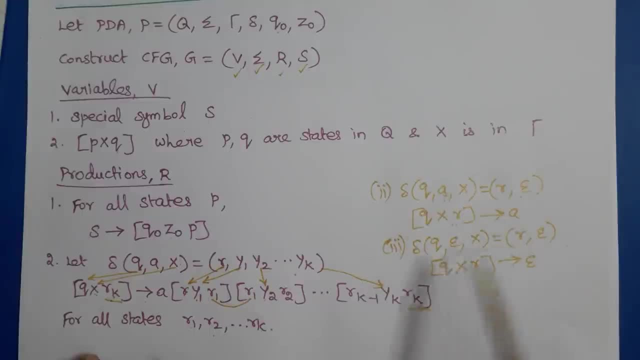 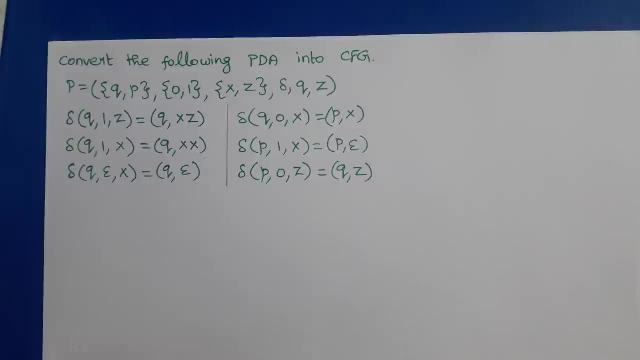 then we need to write only one production like this. then both these two symbols are epsilon. here also we need to write only one production. now we will see an example. so the example is: convert the following pda into cfg. so six triple notation and the six transition functions are given. so now we need to construct set of. 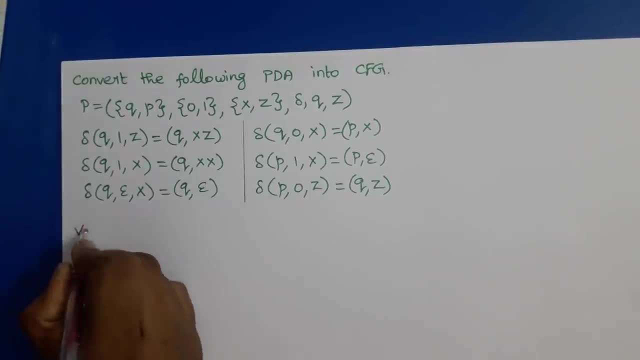 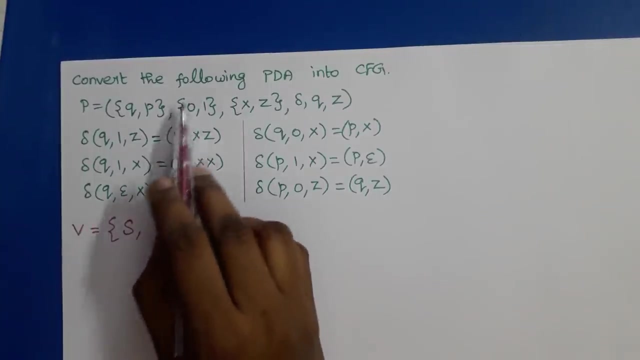 variables for our context free grammar. so the variables v can be written as the start symbol, yes, we need to consider yes as a starting symbol of the grammar, so it is included in v also. then terminal symbols are input alphabet of p. so we have to construct set of variables and 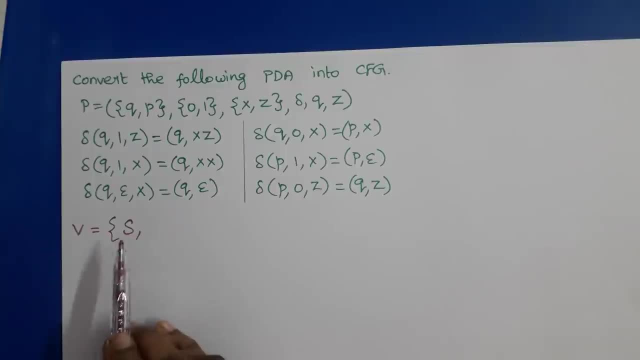 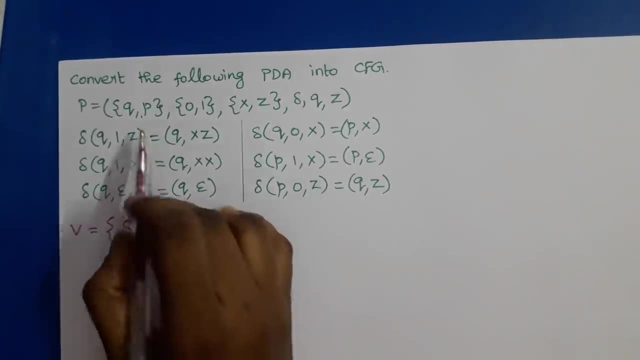 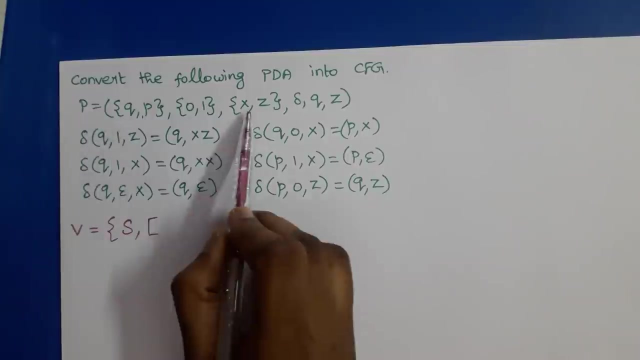 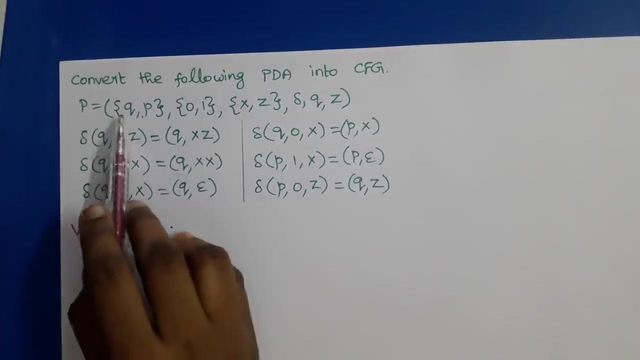 productions alone. so yes, comma, then all possible combinations of a state and stack symbol right. so first, here there are two stack symbols and two states, so we have to first consider the stack symbol in the middle, so we can get four possible combinations right. so q x, q, q x p. then p x, q, p x p. similarly we need to consider z in the middle. so q x, q, q x p. 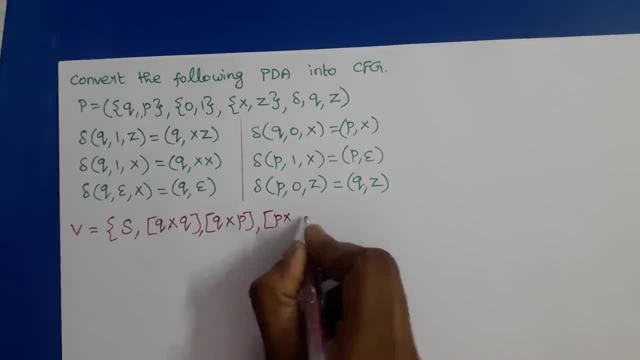 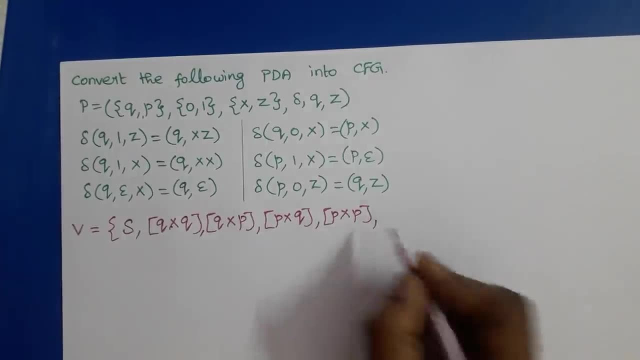 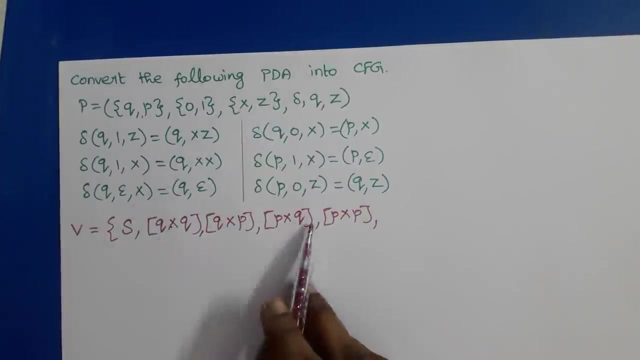 so p, x, q, p, x, p. so there are four states, four, four variables. sorry, four variables we can frame by considering x in the middle. then we have to write z at in the middle. so q, z, q, q, z, p, p, x, p. it is a statement of our main GP k and then again we have cliched name and statements. we can still frame Institute closed, whereas we will get the name gqp into p and the, and we will use in this one also. so let us look at one accessing a number from a given type. as well as this name we will use in this process is a form consisting of a form consisting of ten entities. 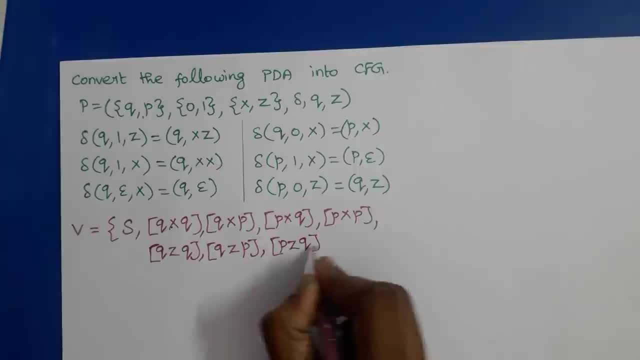 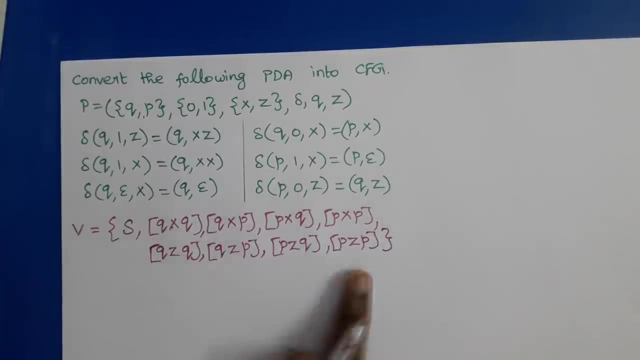 or variables. it has two variables which, at the base, we can name the many that one is. today we are going to wheels go around, so that is what we will write, so here as well. and then one beta will be our with P, Z, Q, P, Z, P. So these are the 8 variables formed for the context free grammar, So these: 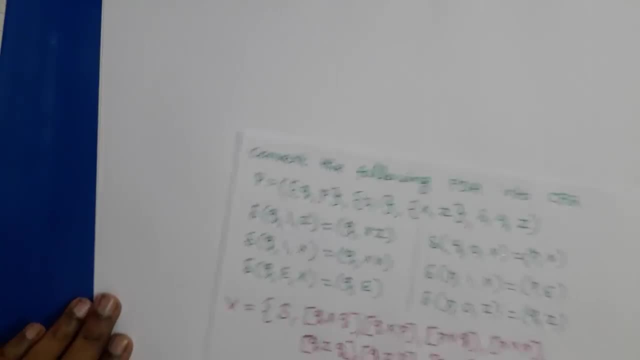 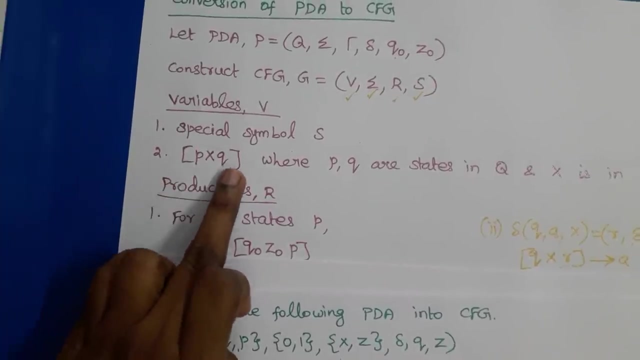 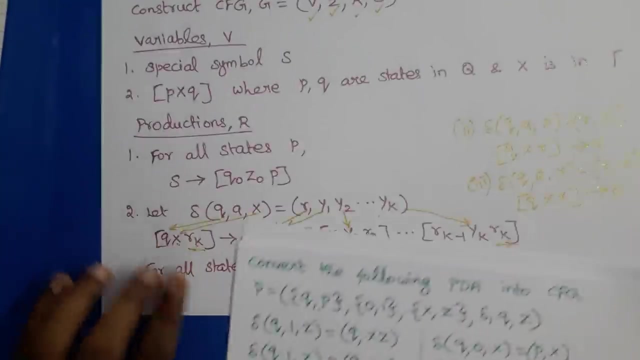 are the set of variables. One is framed from the rule. First rule, yes. Second, we have to construct all variables in the form of P, X, P, where P and Q are the states in Q, X is the symbol in gamma. So we have got 8 different states. Then we have to construct a set of productions. 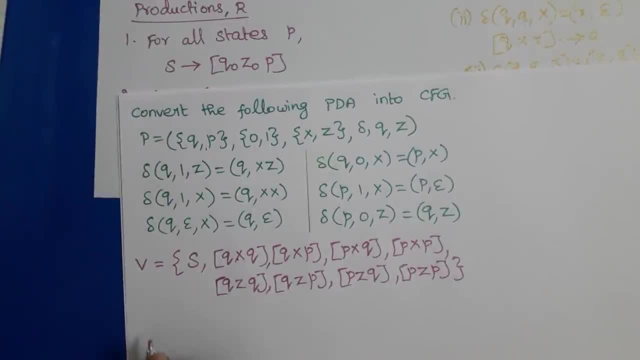 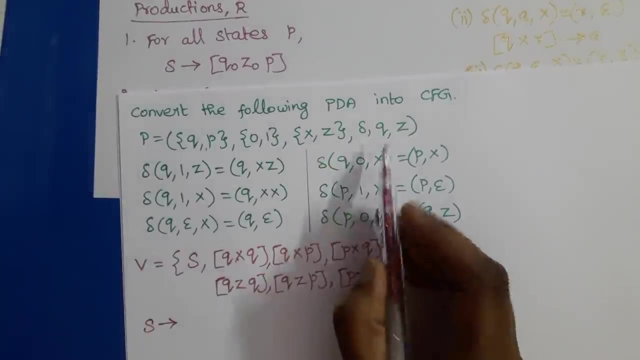 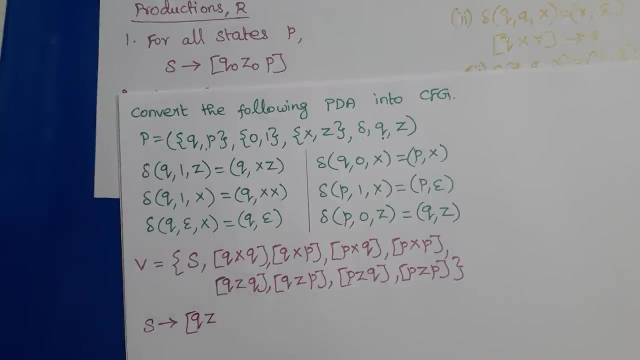 So by following first production, first rule, how to form the rule. The start symbol of the grammar S tends to Q, naught, Z, naught. Here the start state is Q and the start symbol of the stack is Z. So Q, Z, Q, Z, and this P is for all states, So here, 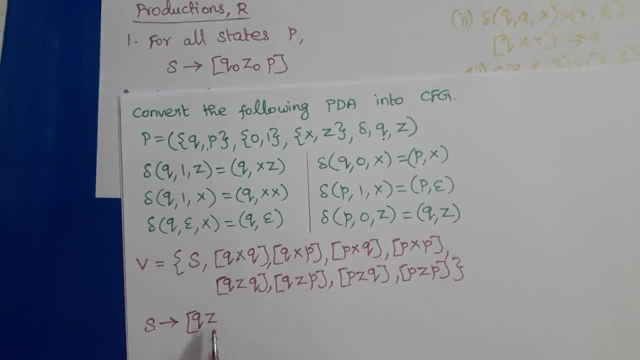 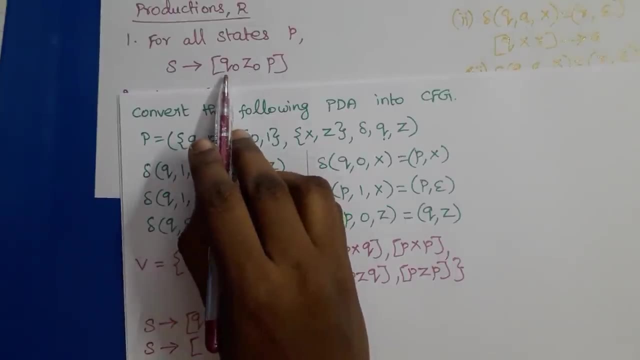 how many states? There are two. So first we have to write Q here, Then one more. production S tends to same Q, naught, Z, naught. So Q Z, here Q, Z, and here we have to write Q, P, right, 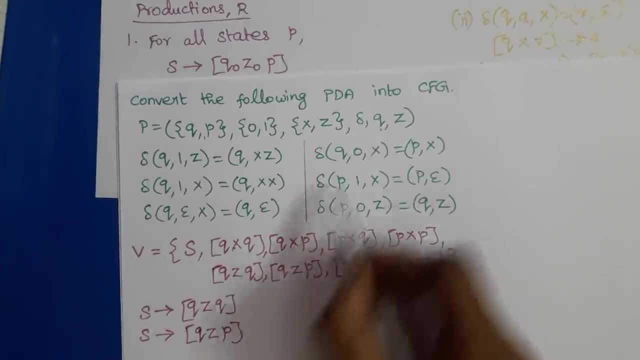 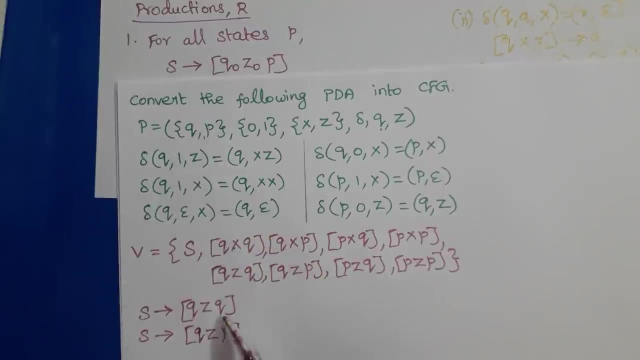 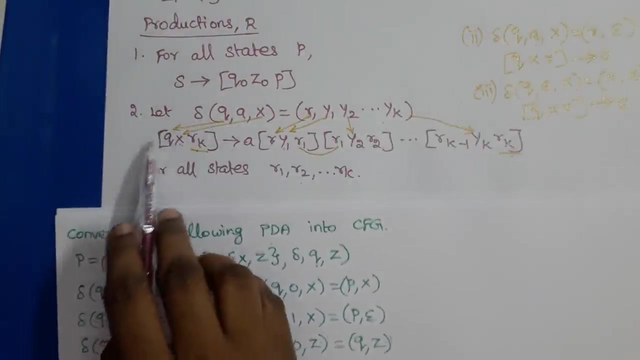 So S tends to start symbol of the grammar, tends to starting state, starting stack symbol, and this symbol must be written for by considering all states, So Q, P. So these are the two rules we have framed, by considering the first condition, Then the second condition. 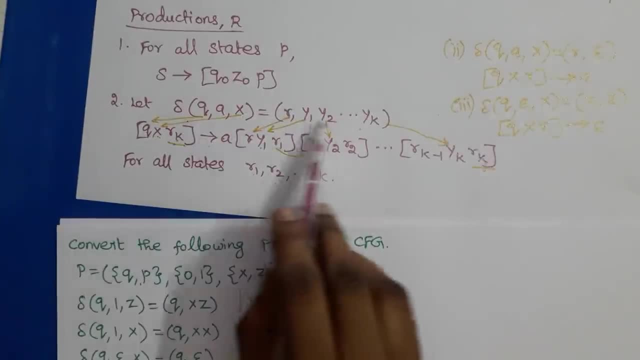 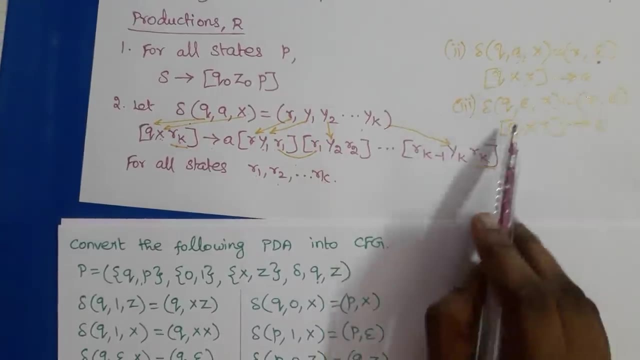 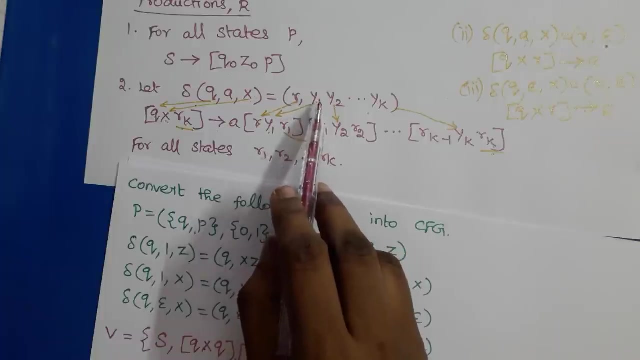 here there are three parts, So it may be a push operation or pop In pop. there are two conditions Here: a terminal symbol may come or epsilon, and sometimes no change symbol. no change operation means here we will have only one non-terminal. So for that also we have to follow this rule. 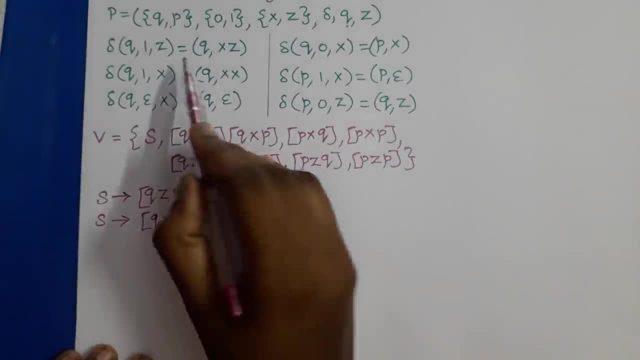 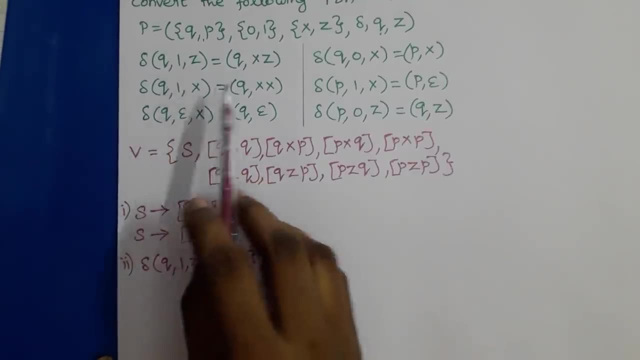 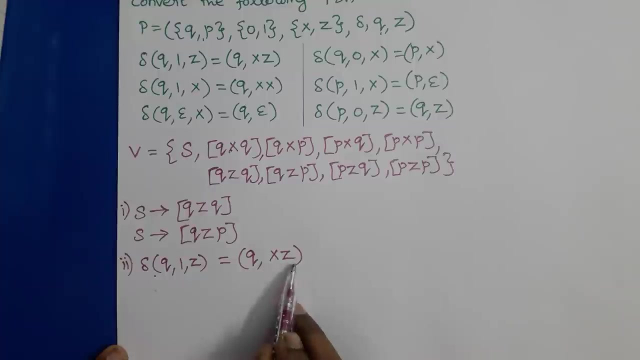 So now we can write. we have to consider all the transition functions one by one and write the rules. So now I have to consider all the transitions one by one. So first I have taken the first transition. So here there are two stat symbols. So we have to write two non-terminals in the right side. So first we have to write this Q. 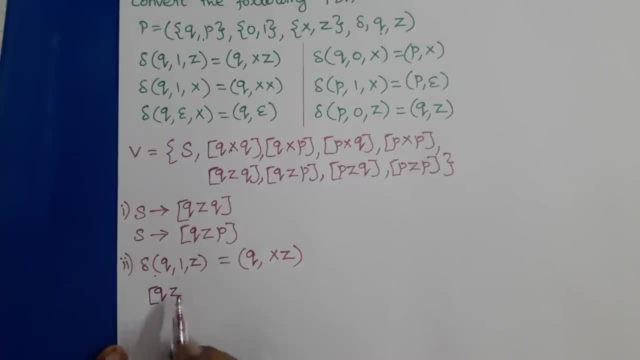 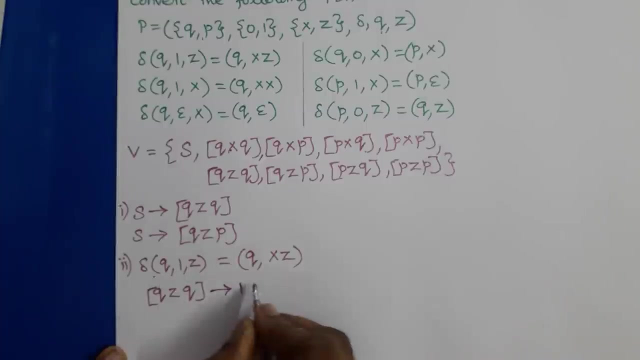 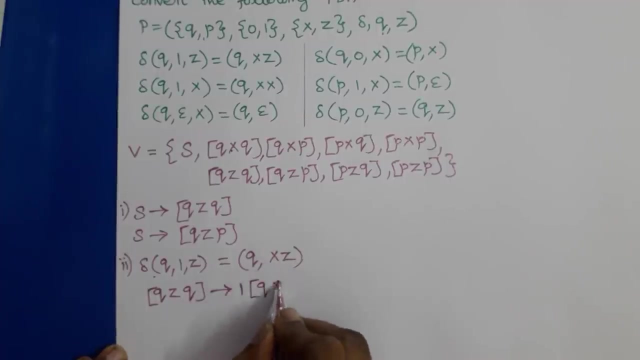 Z, and this symbol must be written for all combinations of the states. So first I am going to write the rule for Q, then I will write the rule for P. okay, so Q Z, this Q implies this terminal symbol 1. and how can I write these two variables? by combining this Q X, Q X, and here also I need to. 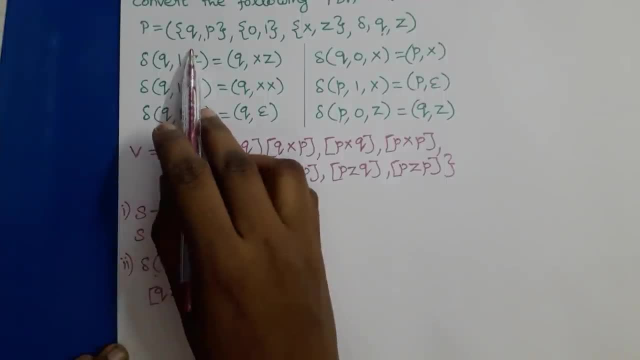 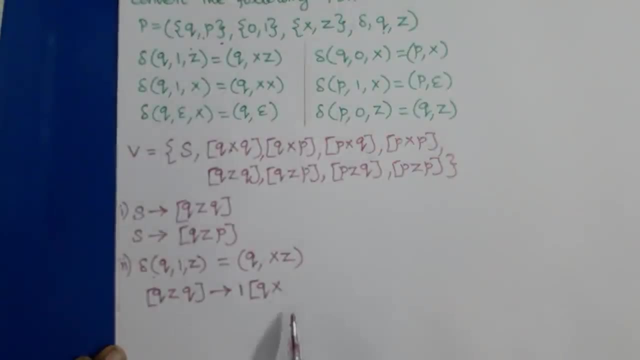 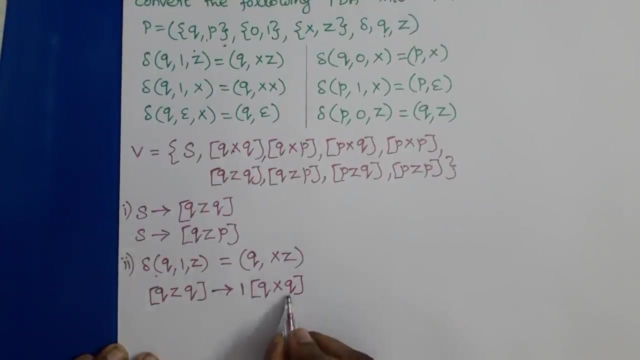 write the state one by one. so first I have to write this rule by writing Q in the middle. then I have to write the same by writing B- sorry P- in the middle. so first I am going to consider Q. so Q, whatever state I have written here, I have to start in the next non-terminal. so Q is written. 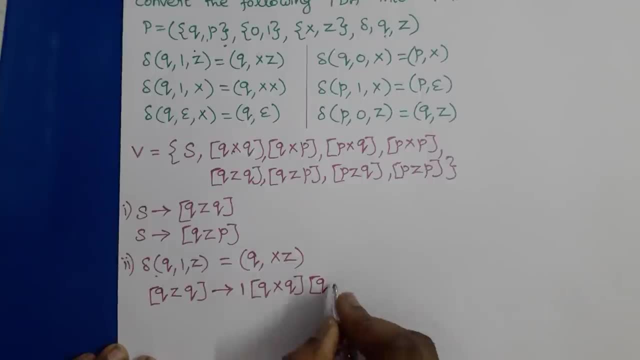 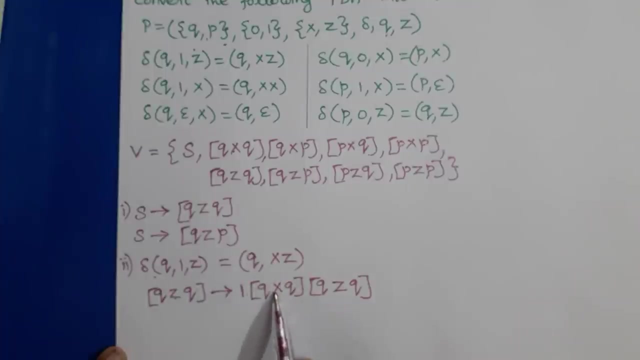 here means, here also I have to write Q, then Z should be written here Z, and this same state should be written over here, so Q, Z. first I am going to write Q here, so Q, Z, Q tends to 1, Q, X, then Q, then the same Q, Z and this Q must be written over here, then the same rule I have to. 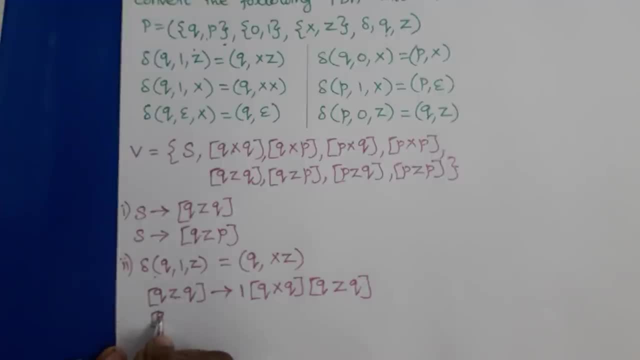 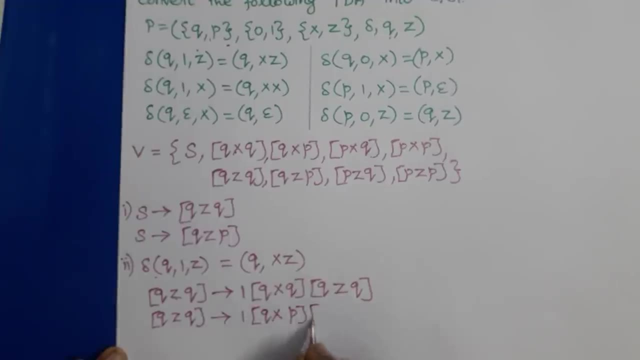 write by writing P in the middle. so Q Z, Q implies 1 into Q, X, P, P, okay, z q. so in the middle portion i have to write p. so now i have written the production, two productions, by considering q here. now i need to write the same two by considering p in the. 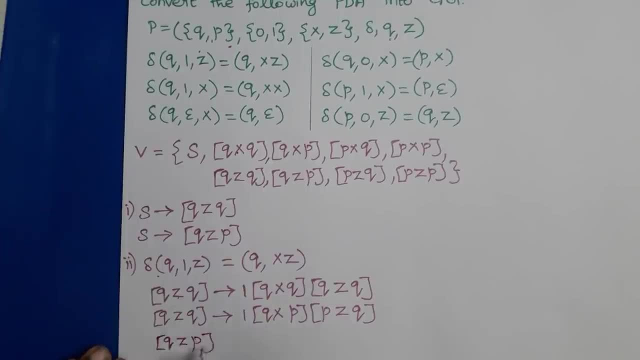 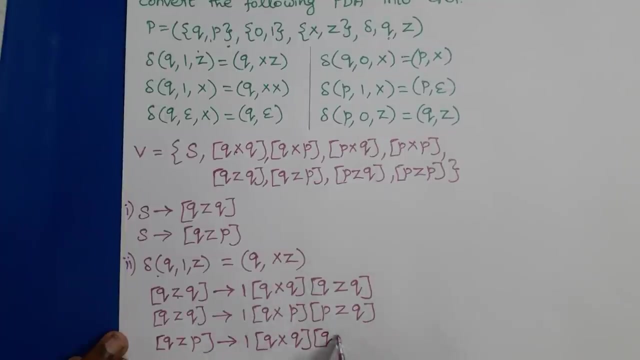 end. so q z p. this q, z and p implies 1 into q x. first i have to consider q in the middle, so i have to start the same q here and this z must be written and this p should be written at end. so now i need to write the same production with p in the middle. so q z p tends to 1. 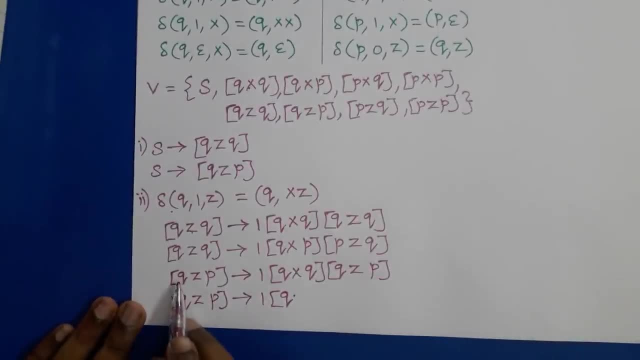 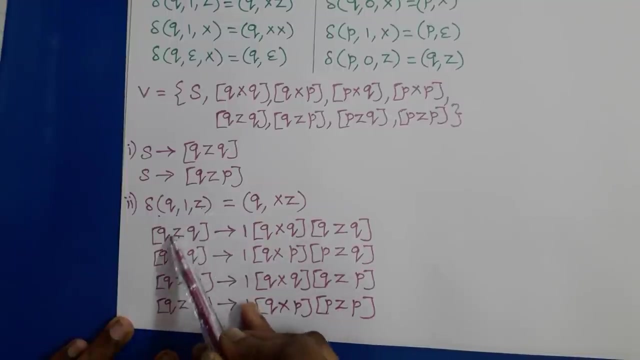 p, q. sorry, q z p tends to 1, q, x, p, p z p. okay, so this state must be written here, then this tag symbol must be written for all four possible combinations. then i have to write two rules by considering q here, then p, because first i have to consider q in the middle portion. 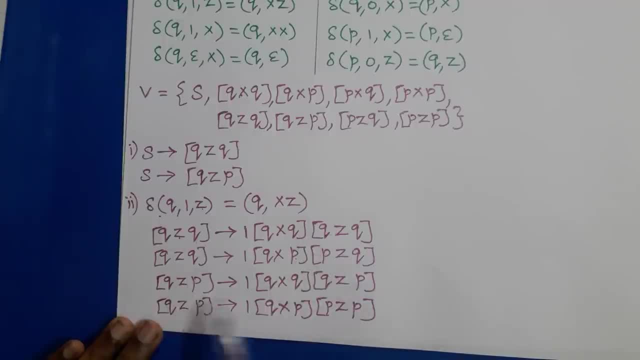 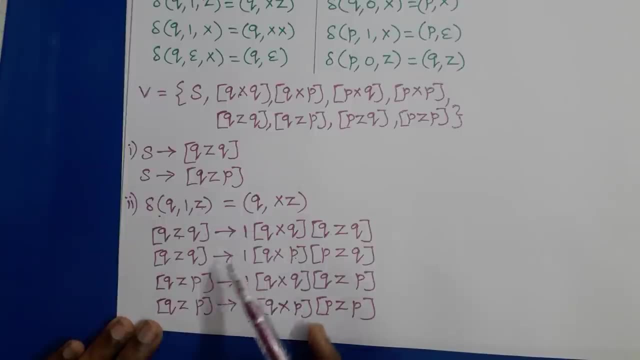 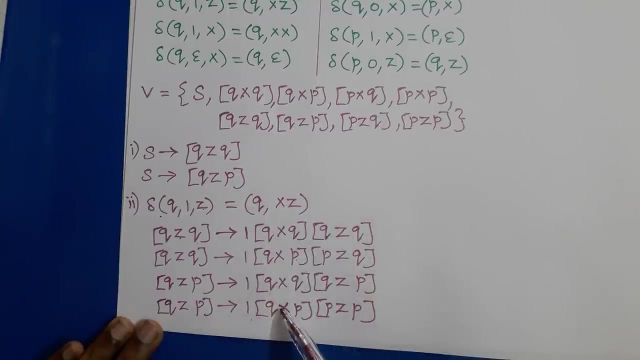 here and p. similarly in p also q and p and whatever state i have, i have written here that should be written at the end and here the terminal symbol should be written, so 1 and this must be the state q and this is x, and here i have to write all. 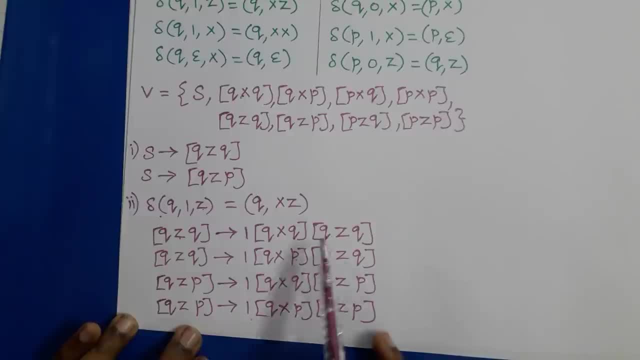 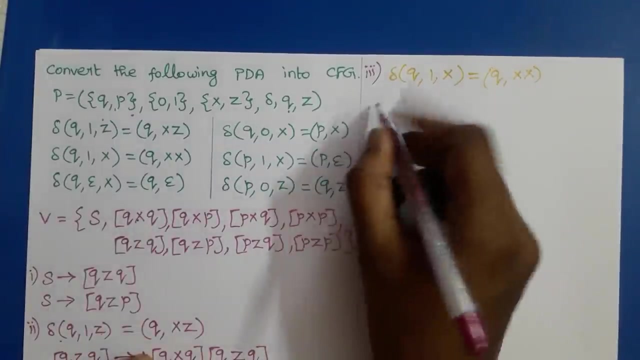 possible. i have already told q q p p, q q p p, and here we need to write this symbol, so z and here whatever state written here, that should be written over here. so q q p p. now i have taken the second, second transition, so here also there are two symbols here, so we. 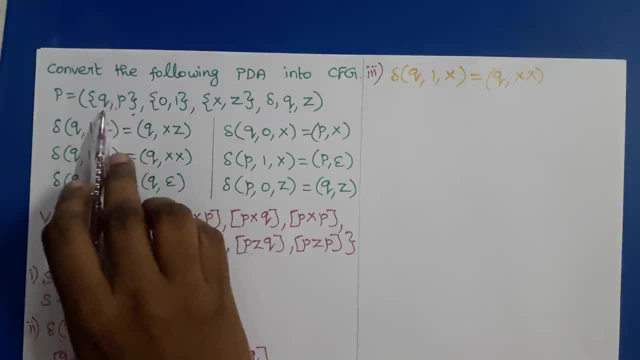 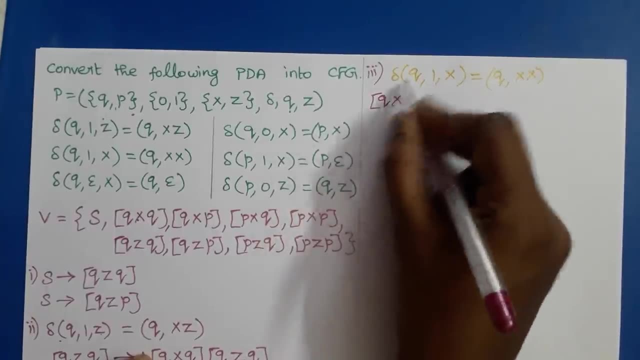 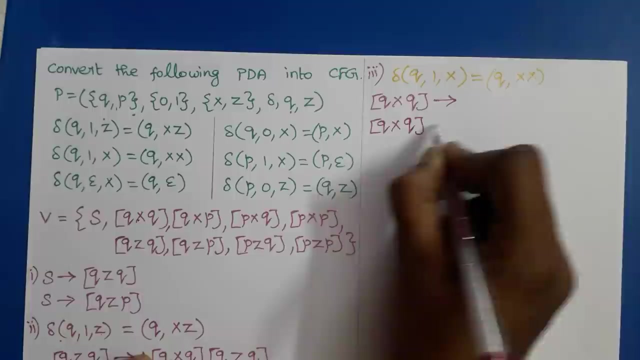 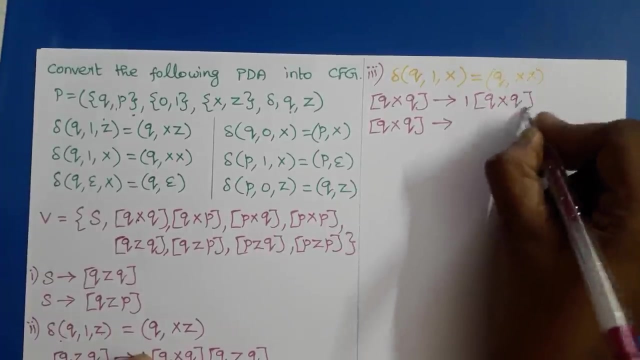 will get four possible combinations because it has two states, so we will get four possible combination. so q x, q x. first i am going to write for q. so there are two rules: q x, q, so one this q x. first i am going to introduce q here, then the same q. the second symbol is also. 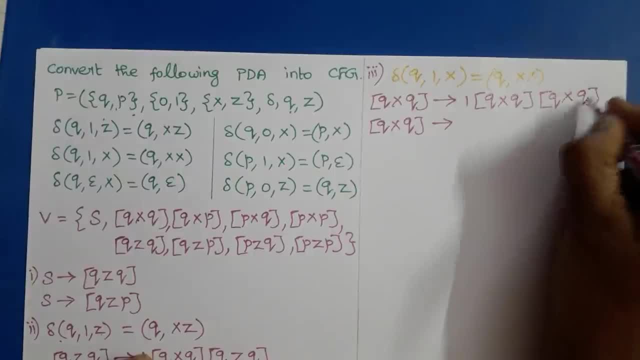 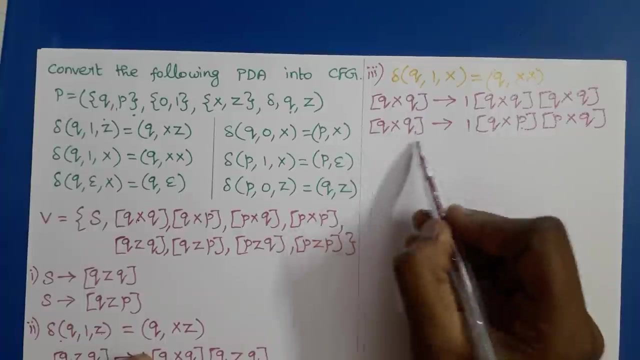 x here. so x and this q should be written here. similarly, one q, x. now i need to write for q and this q should be written here. so x and this q should be written here, p in the middle. so p x, this q. now i have to write the same, but instead of q i have to write 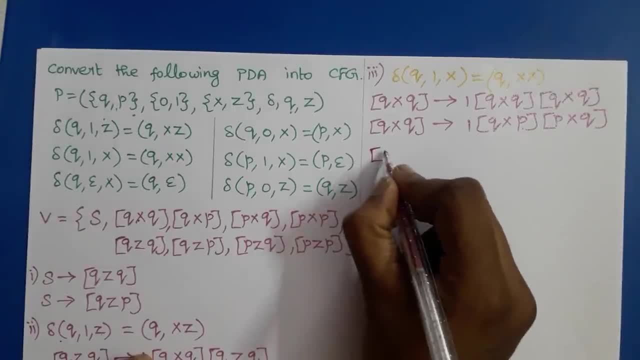 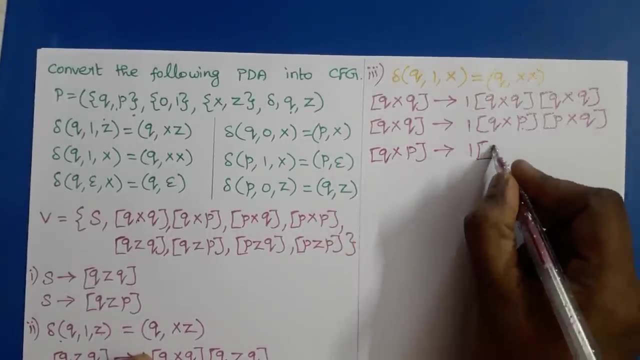 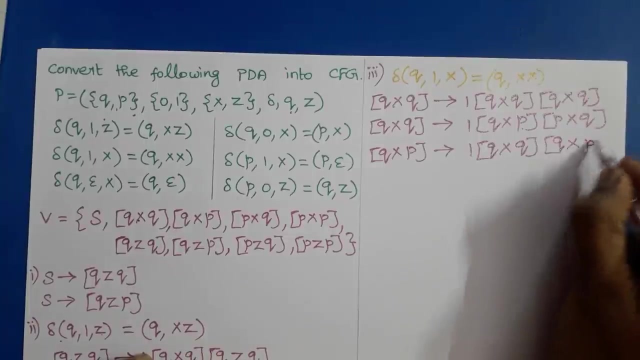 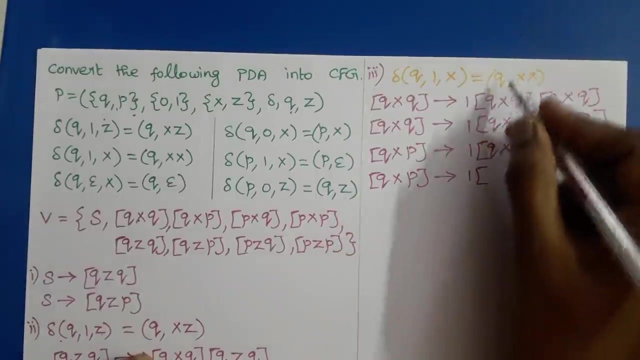 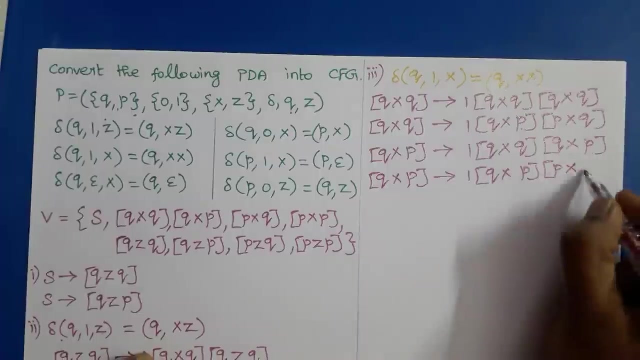 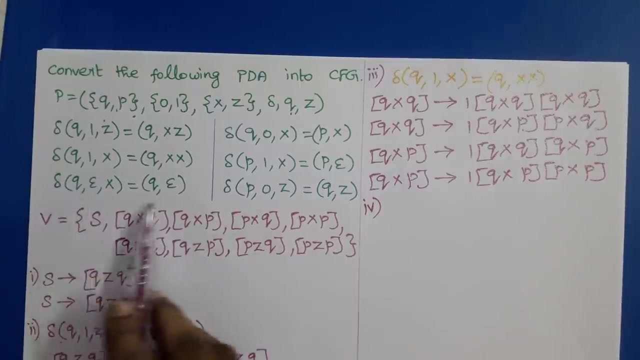 p. so these two symbols must also be changed. so q x p tends to 1 q x q. the same q x p. then q x p implies 1 q x. here i am going to write p, p, x, this p. so now fourth one. fourth, fourth rule is a third transition function, because i have written, i considered this as: 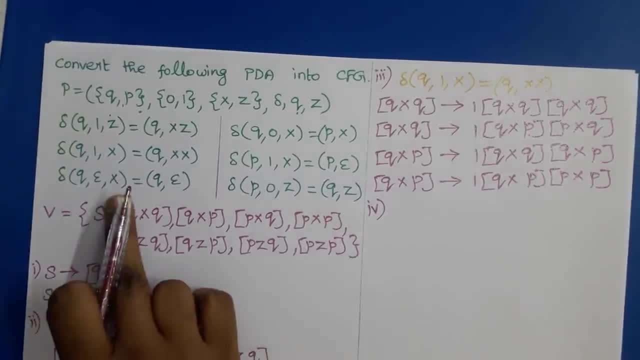 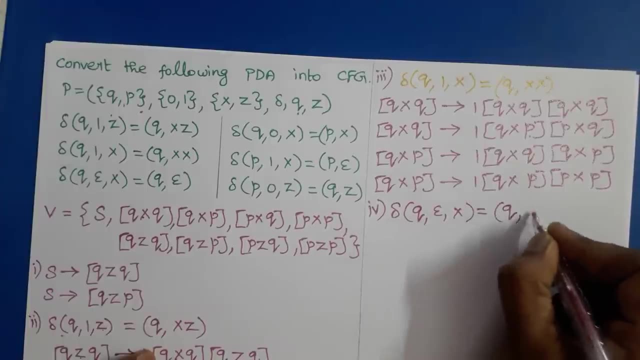 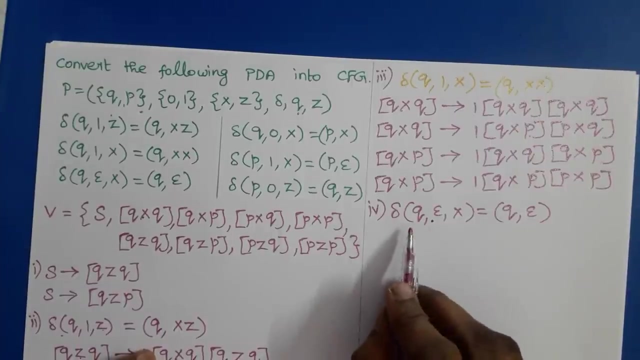 first step. so fourth set of productions can be formed from the transition function, so del of q comma epsilon, comma x equal to q comma epsilon. so here epsilon and epsilon came. so we need: we will get only one production, so q x q. this is a variable, so q x q. 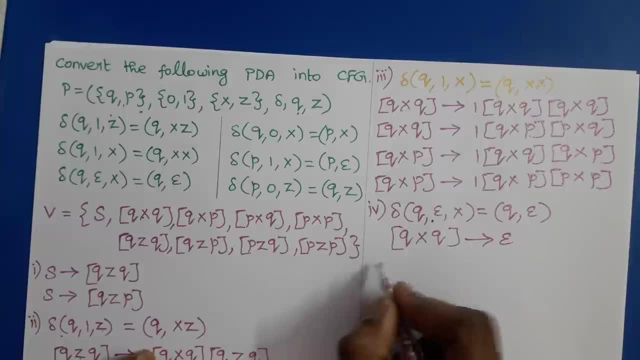 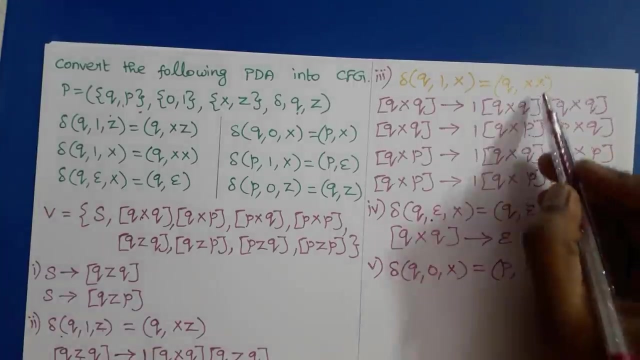 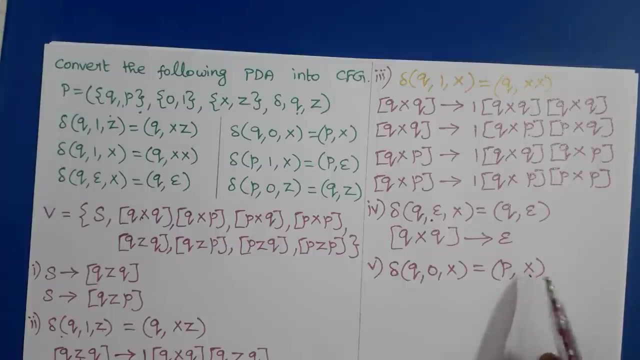 implies epsilon. then the next one is this rule: so del of q 0, x equals p comma x. so here we have got one symbol. okay, in these two rules two symbols, but here one symbol is. one symbol is the stack symbol. that is no change operation. this x replaces x. on. 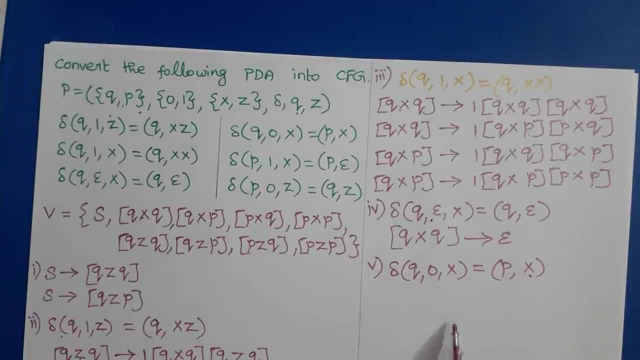 top of the stack. so we will get two productions here, okay, one with q, another one with p. so i have to write q- x. first production i need to write with q. here implies this 0, p, x, and this q should be written at the end. then another production: i need to write q- x and i have to consider p here. 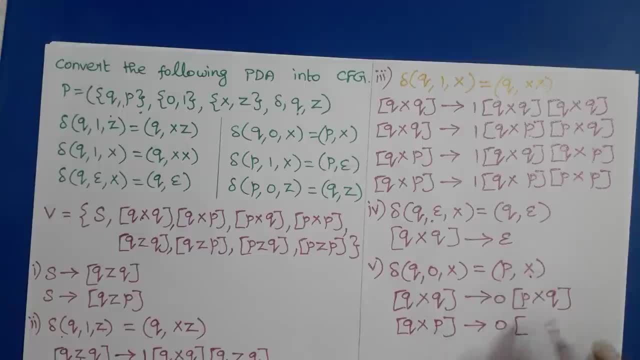 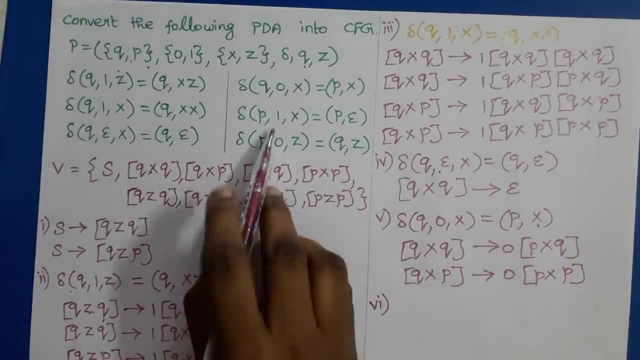 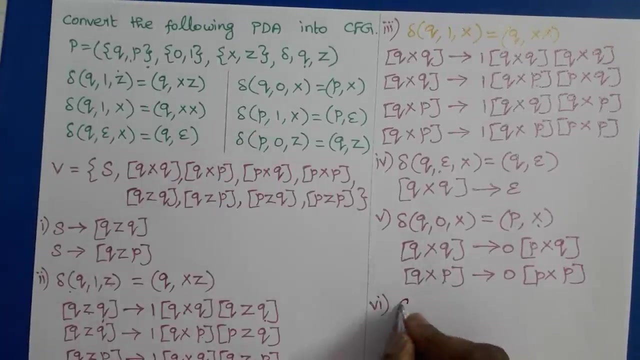 implies this: 0 p x, and this p should be written over here. okay, then, sixth rule is- i need to write this, sorry, this one- so del of p comma 1 comma x, equal, equal to p comma, epsilon. so here epsilon is coming, but here the terminal symbol. but in this case also, we will have only one rule. so p x, this p. 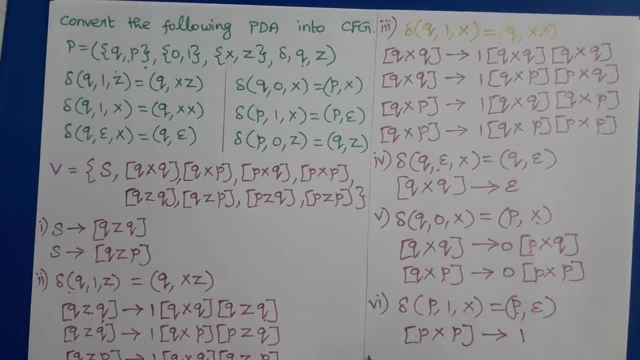 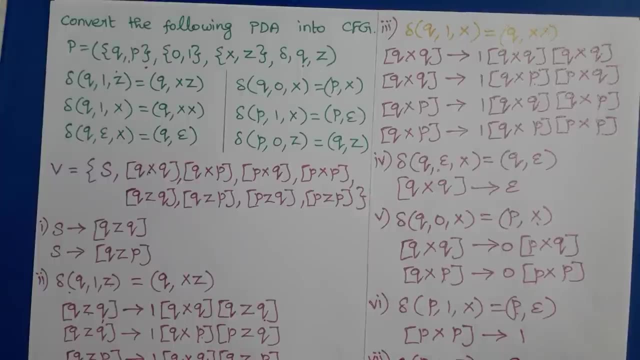 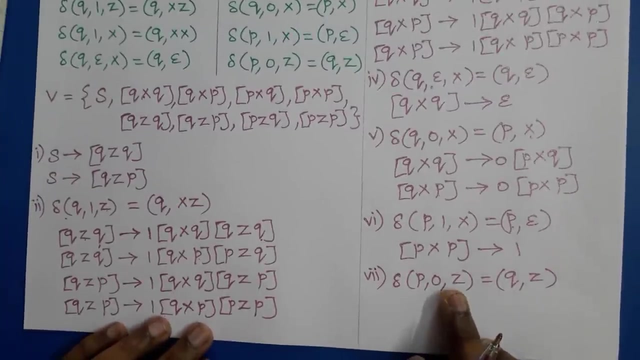 implies 1, then the final function is del of q x and this p implies 1, so del of q x and this p implies 1, so del of p comma 0, comma z equal to q comma z. so here also one non-trimmable, no change operation. 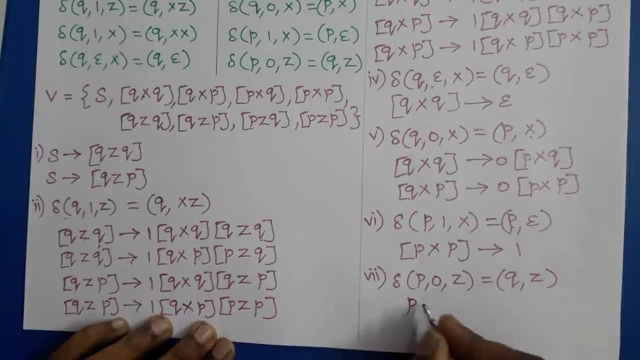 this z replaces z on top of the stack, so we will get two productions like this. so q uh, p z. i have to consider q first, so p z q tends to 0 q z. this q at the beginning, so it has a有一 and we have this one which is some basis point. so so there's only a base coming in first line. so some basis points below that's left by the middle minus. that gives us just two: ה�qualified right and the anymore second variable before got to the first line: in猶 employed here. so there's a base 문제 marks here. so that's the outcome if we get the gratefulness؟. so it is what we have, and that's a difficult one: capacityог that that two produce times and that two Ensure that we can say e and b are similar to b, and this is another probability that we have. we shall not tend to alright, mark.